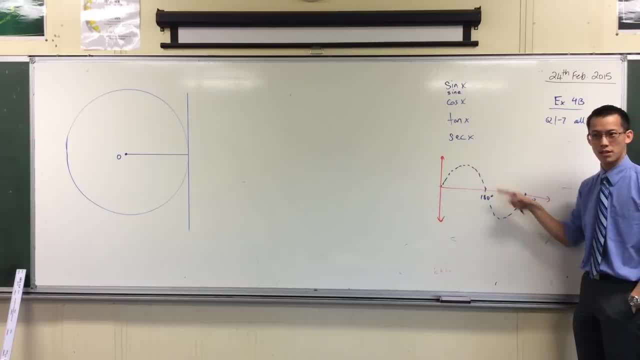 Okay, so sine, its name comes from this shape, which comes from: if you were to put in, if you were to test out all of the values for all of these different angles, then these are the sines of those angles. okay, 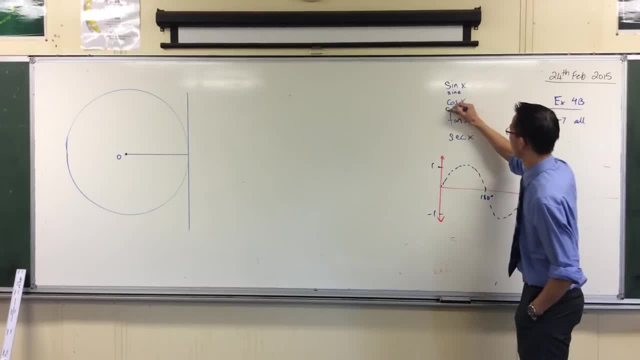 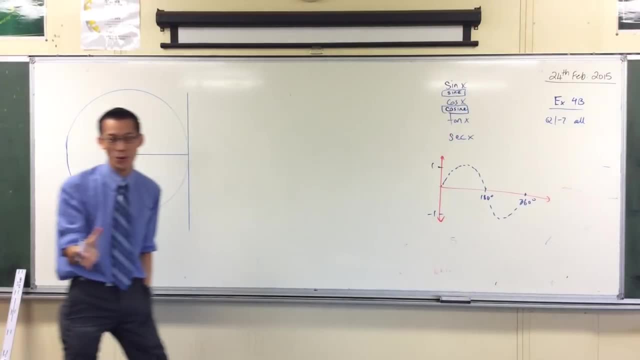 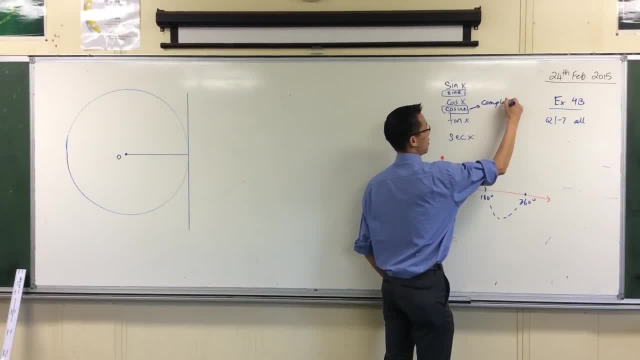 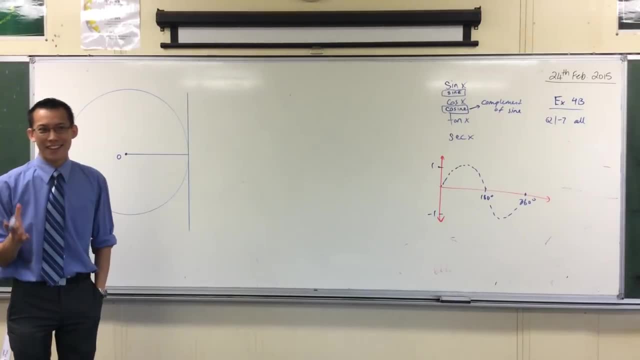 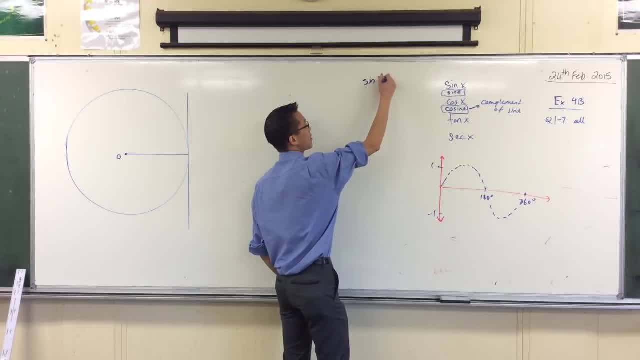 So what does this mean? What does this mean If you take an angle like 30 degrees? we know what sine 30 is equal to. We were just talking about it, right? Well, whatever it's equal to, It will be equal to the cos of the complement of that angle, right? 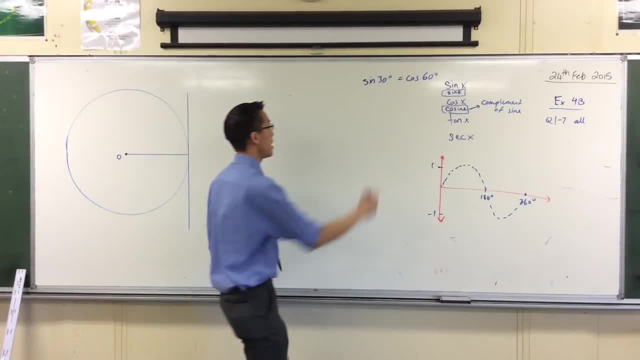 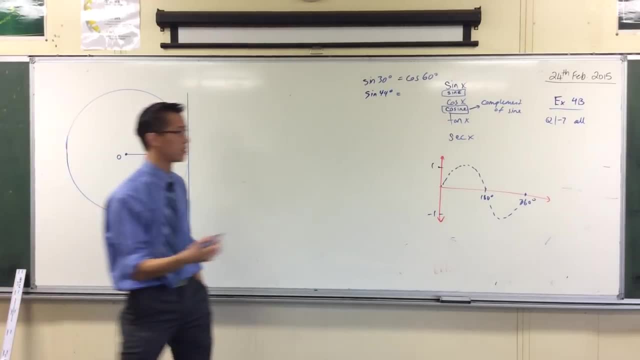 And you can go ahead. you can redraw the triangles to test it right. In the same way, if you take any angle you like, then it's cosine right. The cosine of the complement of that angle will be the same. So that's where it comes from. 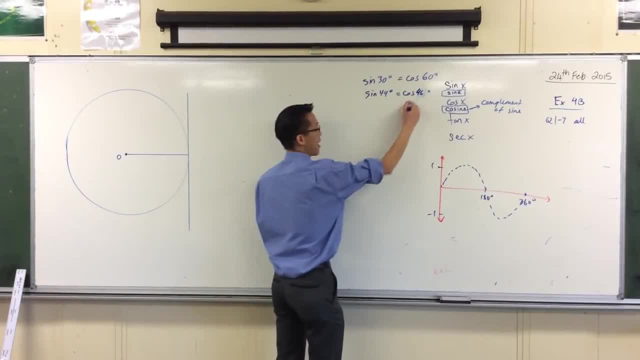 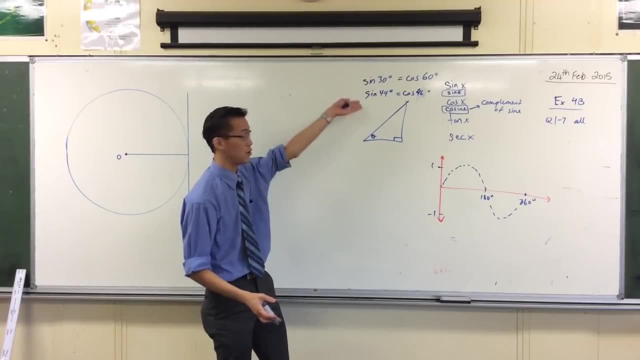 You might think, well, is it really that useful? Well, by the way, you can see why When you draw the triangles, right, If you make a theta down here, You don't know what theta is. It could be 30, or 44, or whatever you like. 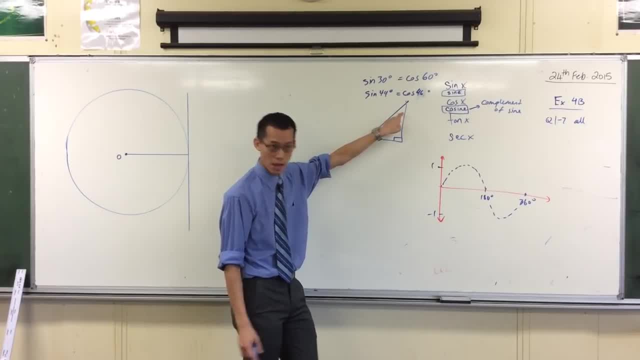 Then clearly this opposite angle over here is going to be 90 minus theta right. So right from there you get your definition. okay, If I call this, let's see well, our traditional names for sides in a right angle triangle right. 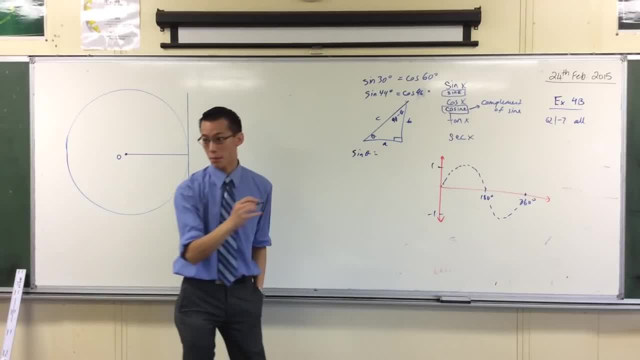 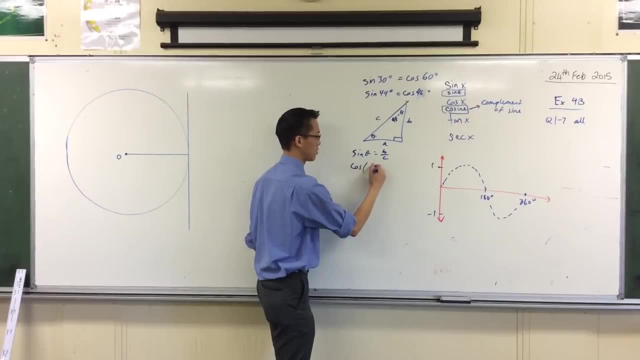 If I take sine theta, that's opposite on hypotenuse, which is B on C right, And if I take cos of the opposite angle, Cos of 90 minus theta right, That's going to be adjacent on hypotenuse. 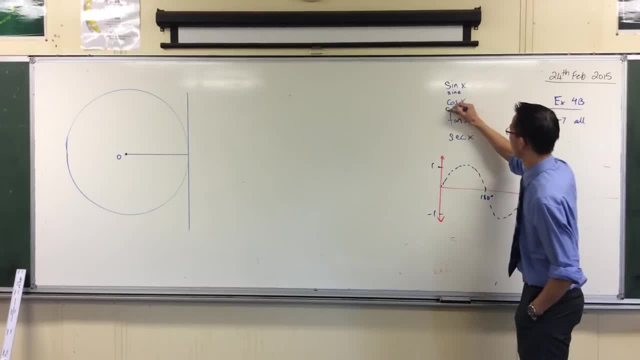 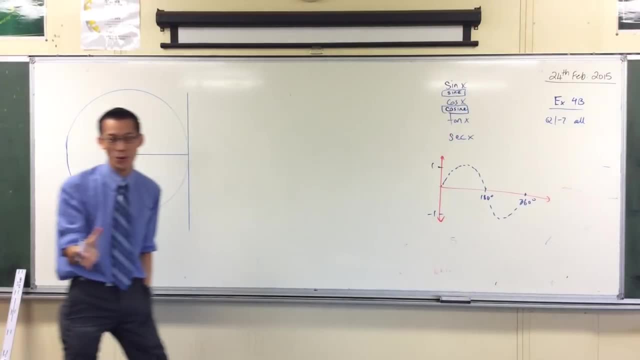 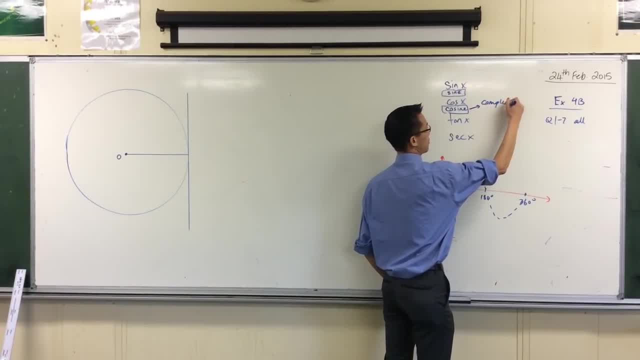 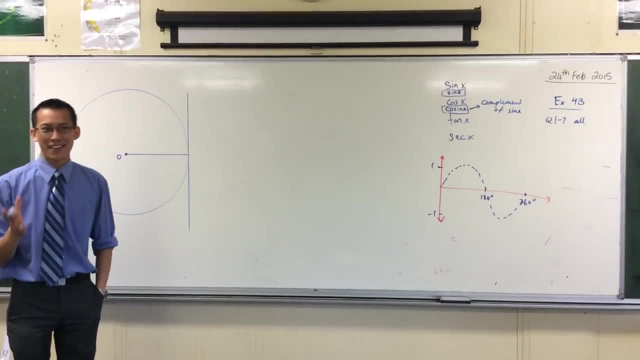 Co, Co, Co, Co, Co Co. So this just means the complement of sine, Complement as in. complement as in adds up to 90 degrees, rather than complement as in. hey, nice haircut, okay. So what does this mean? 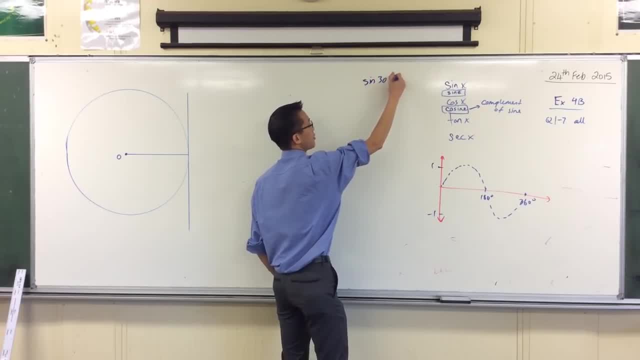 What does this mean? If you take an angle like 30 degrees, we know what sine 30 is equal to. we were just talking about right. Well, whatever it's equal to, It will be equal to the cos of the complement of that angle, right. 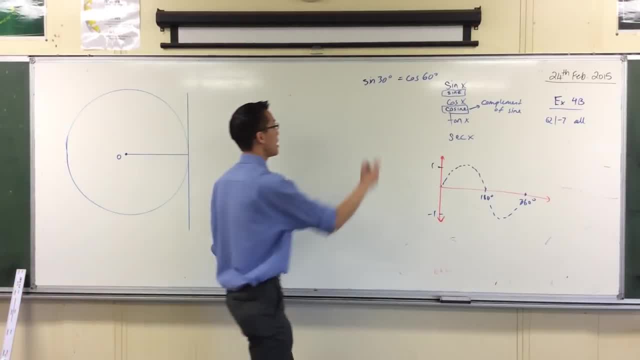 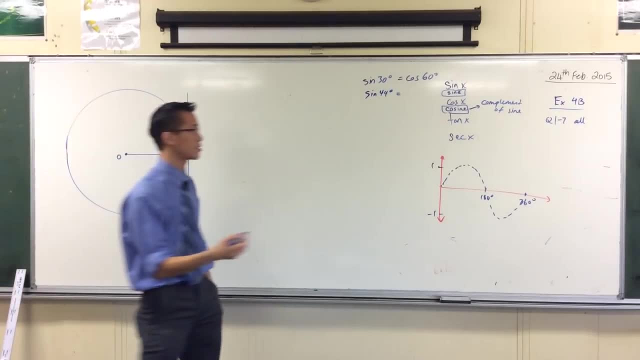 And you can go ahead. you can redraw the triangles to test it right. In the same way, if you take any angle you like, then it's cosine right. The cosine of the complement of that angle will be the same. So that's where it comes from. 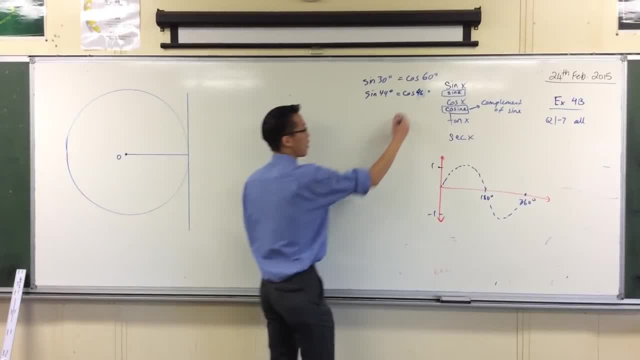 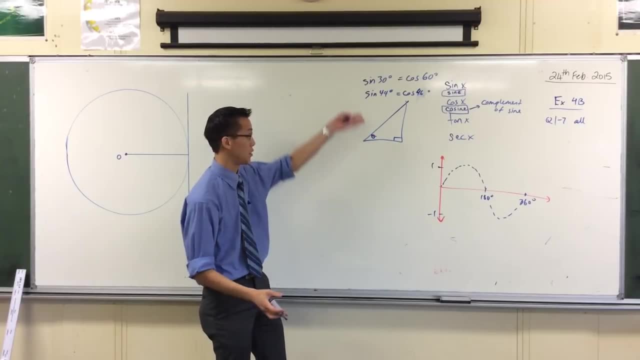 You might think, well, is it really that useful? Well, by the way, you can see why when you draw the triangles: right, If you make a theta down here And you don't know what theta is, It could be 30 or 44 or whatever you like. 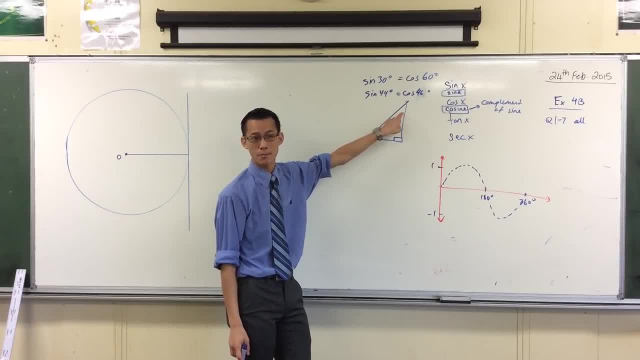 Then clearly this opposite angle over here is going to be 90 minus theta. all right, So right from there you get your definition. okay, If I call this, let's see well, our traditional names for sides in a right angle triangle right. 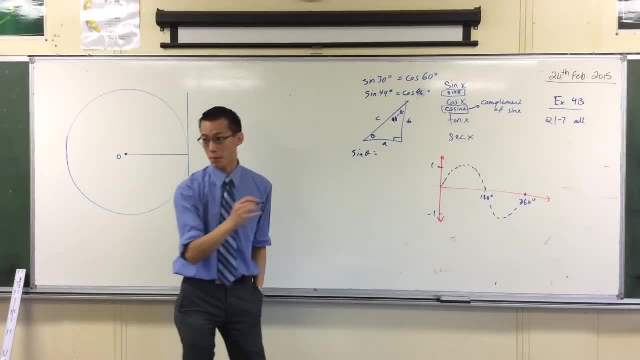 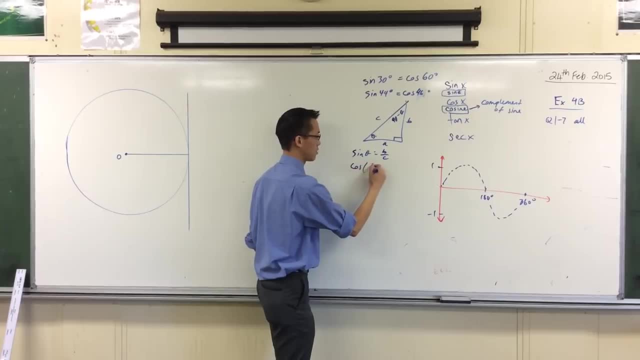 If I take sine theta, that's opposite on hypotenuse, which is B on C right, And if I take cos of the opposite angle, Cos of 90 minus theta right, That's going to be adjacent on hypotenuse. 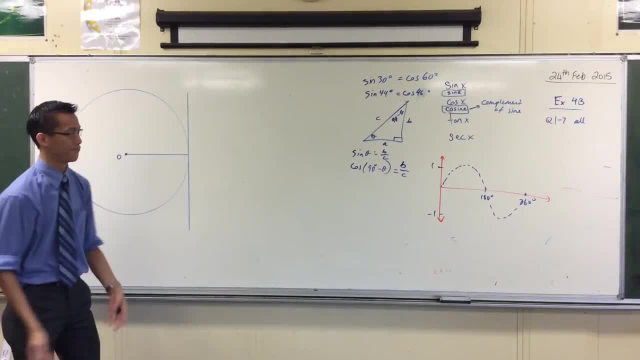 So that's why they're the same. Okay, so there's sine, there's cosine. Where does tan come from? Or, more specifically, where does tangent come from?